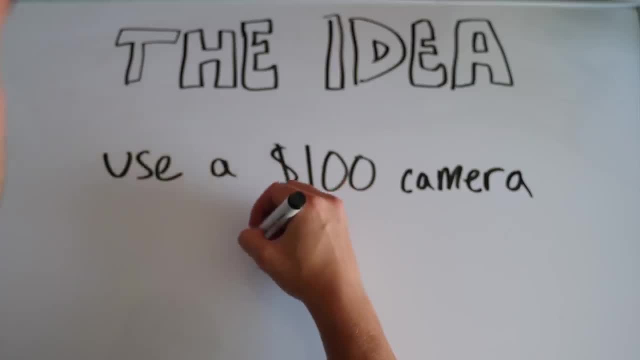 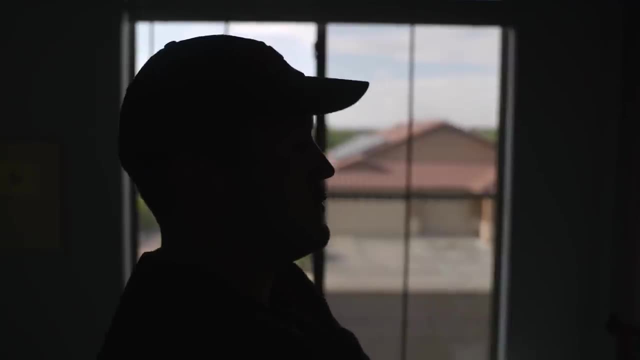 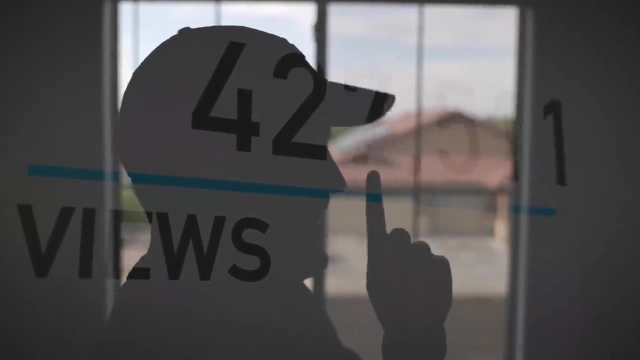 And so this was the idea. I thought it'd be awesome to shoot a YouTube video for Think Media using this camera and see if anyone notices If this goes as good as possible. the video does well. no one notices the camera quality and I can finally tell people to stop giving me the excuse. 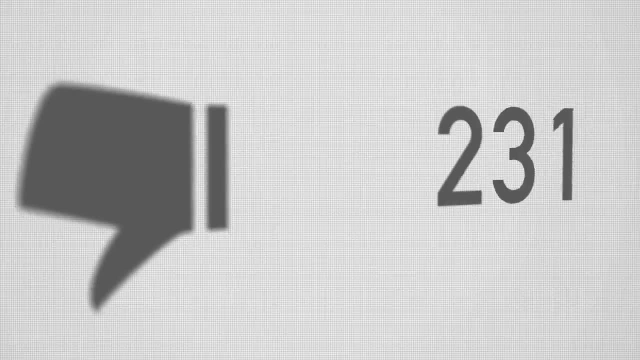 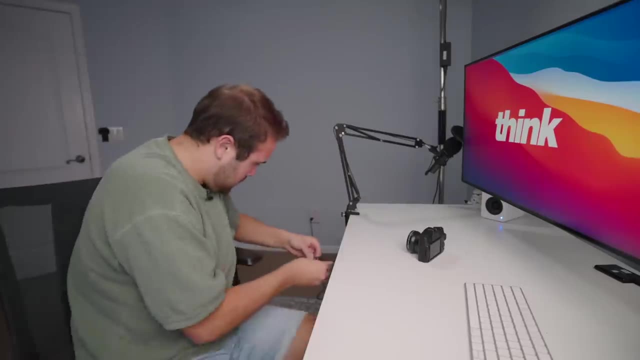 that your camera isn't good enough. If this goes badly, the video flops, the comments rage with 2 million angry subscribers and my boss fires me And, honestly, I was really excited until I looked at the footage for the first time. 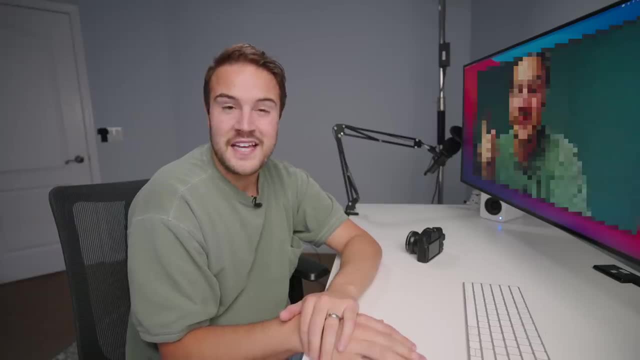 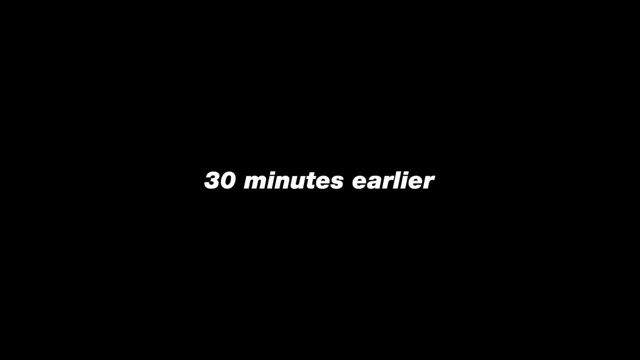 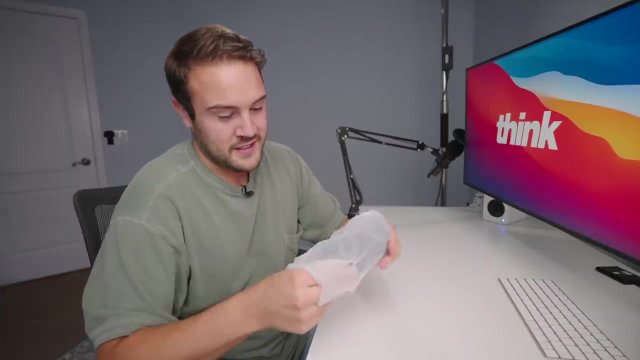 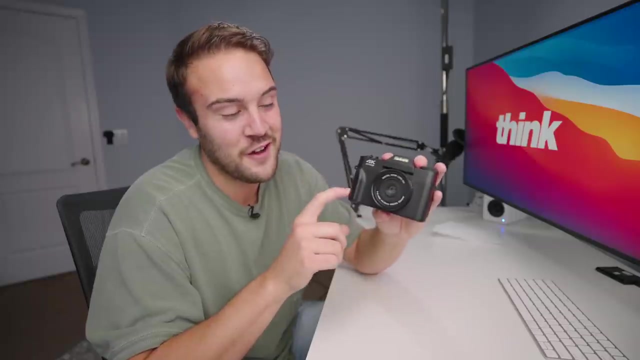 and realized that this was probably a terrible idea. So let's go back to when I was still optimistic about the experiment. It's a $100 camera. As long as the camera works and it's decent, then that's okay. Okay, Now, before I turn this thing on. 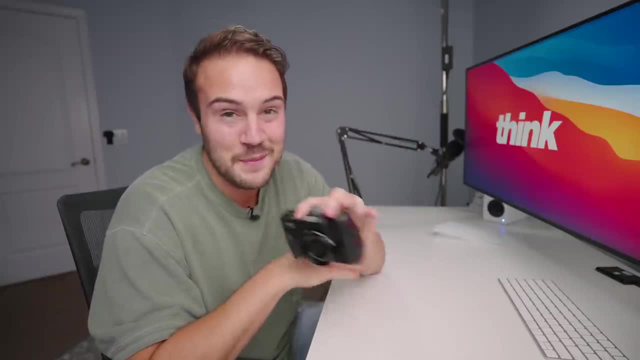 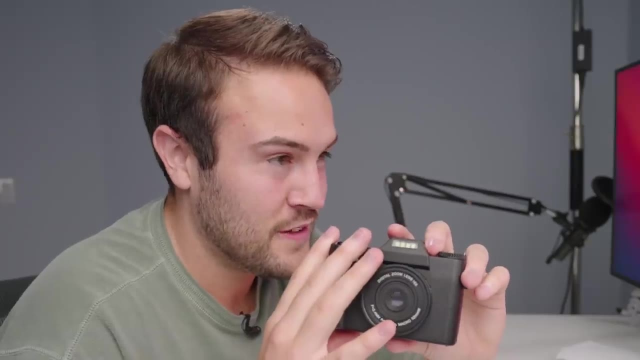 guys, I've already committed to this, So whether it's decent or it's absolutely terrible, I'm gonna have to use this camera to shoot my YouTube video and post it. We got a power button on top, so let's hit this and see if it turns on. 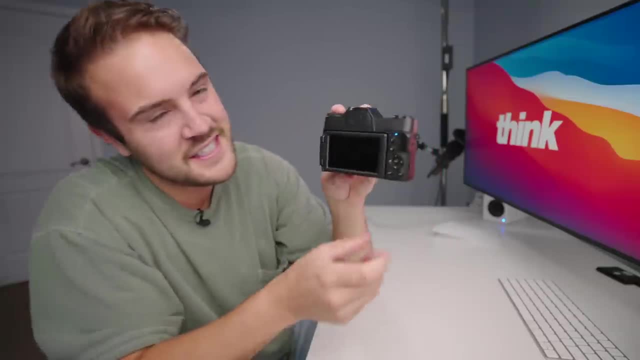 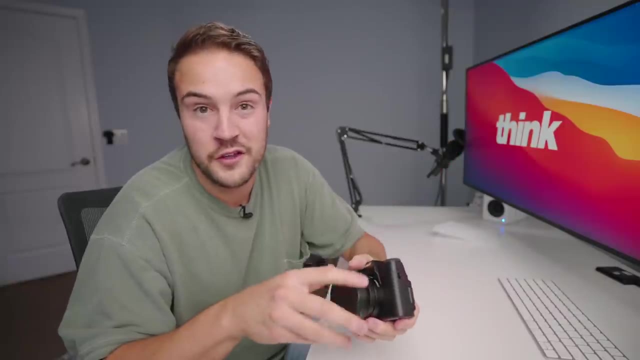 Please turn on. Maybe you have to hold it down. Oh, there it goes. I see a light. Welcome Guys. I'm so excited about this. Ooh, Let's throw this wide angle lens onto the camera and get the full effect. 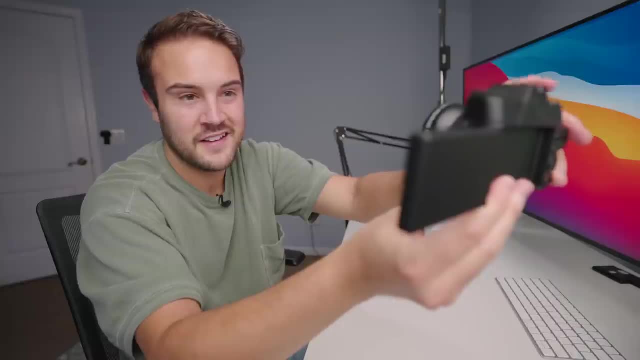 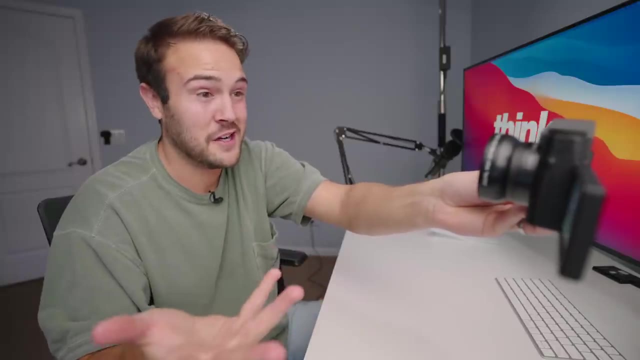 This thing has a front light. Are you kidding me? All right, here is the first test on the $100 4K camera on Amazon. Here is the moment of truth. All right, here is the first test Ugh The $100 4K camera. 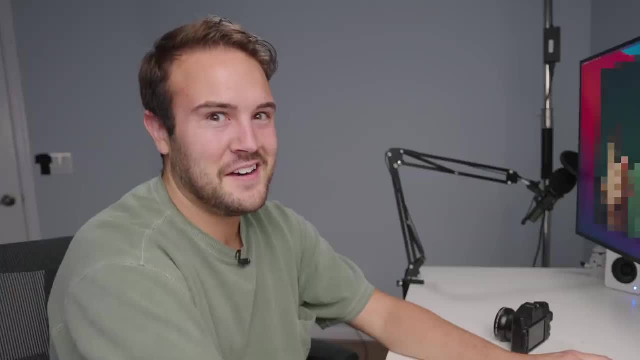 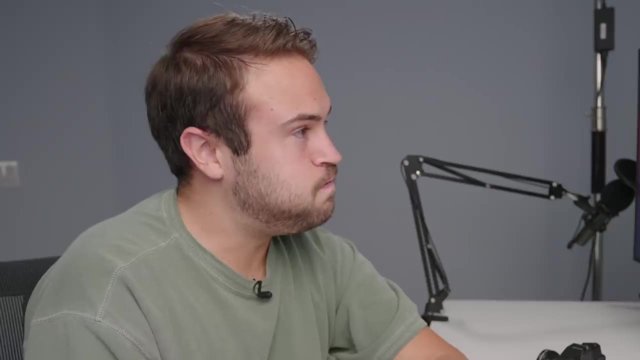 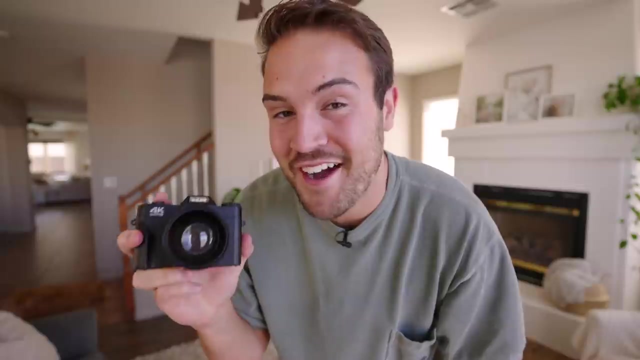 The $100 4K camera on Amazon. Ugh Why, This was probably a terrible idea. Before I take some test footage with this thing, I'm gonna show my wife my brand new camera and I'm gonna see how much she thinks this thing costs. 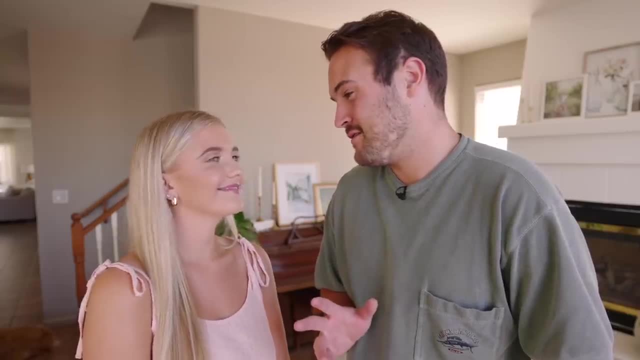 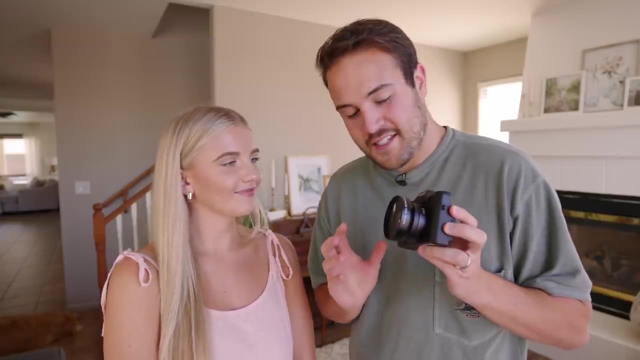 So I wanna show you my brand new camera. Are you ready for this? Yes, You excited. Yeah, I'm excited. Here it is. I want you. It looks so vintage. I want you to guess how much. I want you to guess how much. 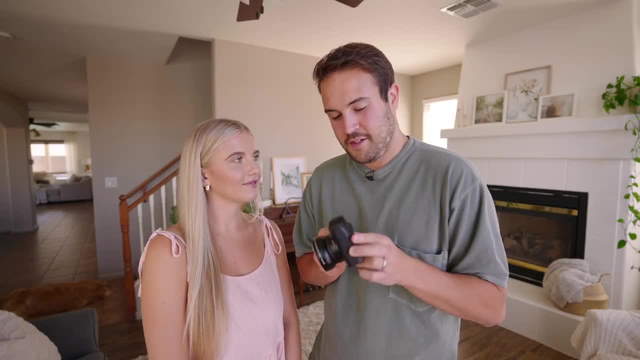 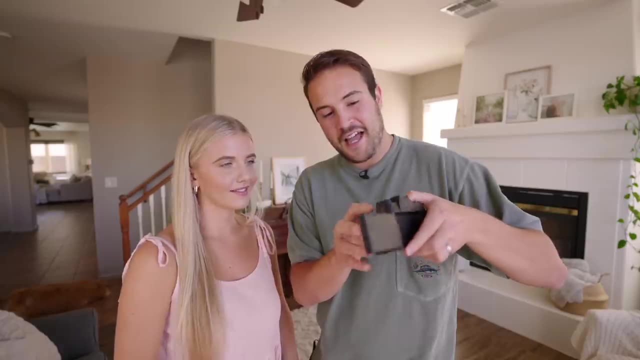 this cost Um $300.. Here, take a look at it. It's got a flip-out screen, but you can't like tilt it any other way, It just flips right back like that, Got a flash. It shoots 4K video. 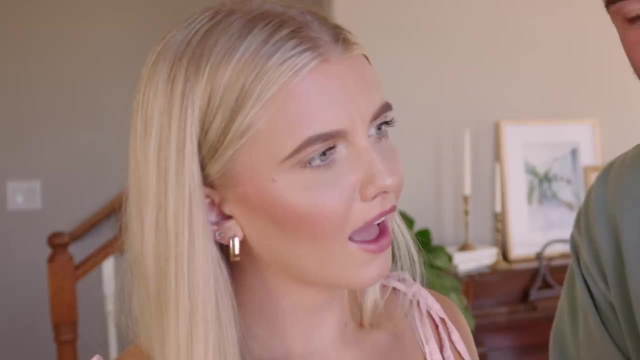 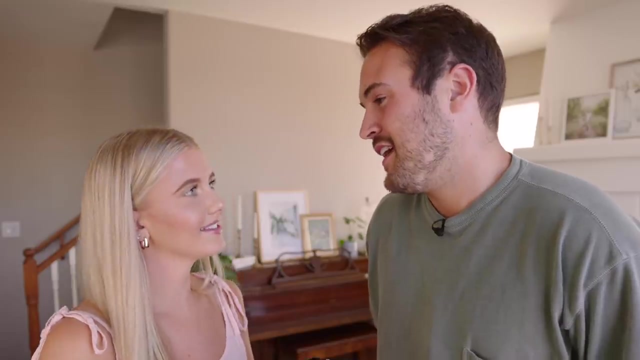 This is a wide angle like lens adapter. You think $300?? Yeah, cause it looks cheap. I love to say that Yeah, it is cheap. Yeah, that's my guess: $100.. Seriously, I don't know. Also, I'm shooting my next YouTube video with this camera. 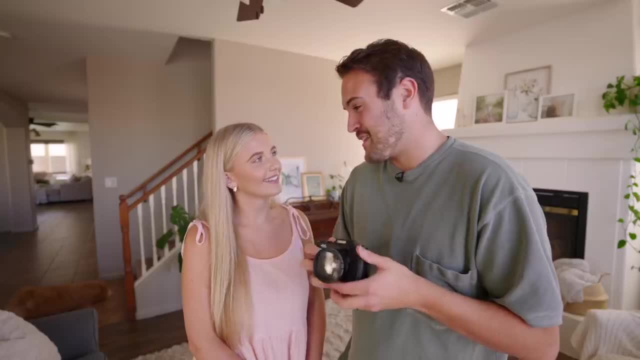 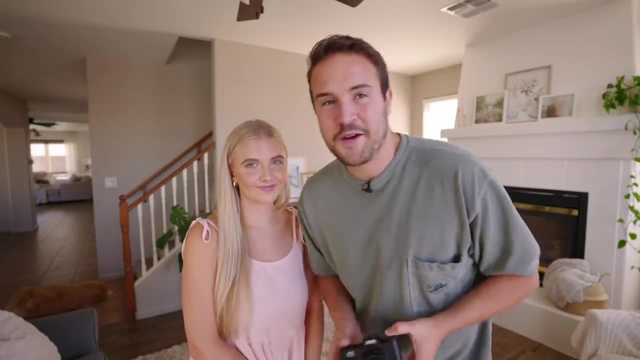 Without telling anyone. Are you just gonna see? if people notice? That's exactly what I'm doing. Hopefully they don't realize Or they're like: what camera is this? Probably not. Let's test this thing out. You wanna say something? 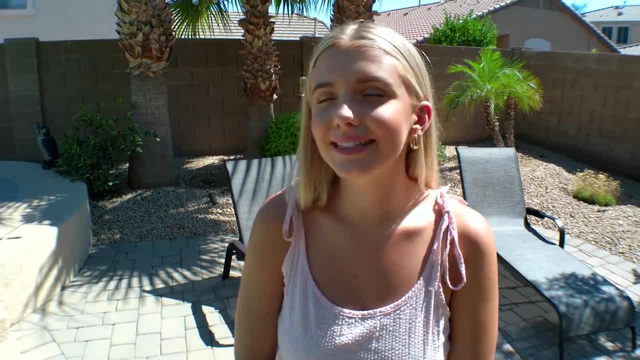 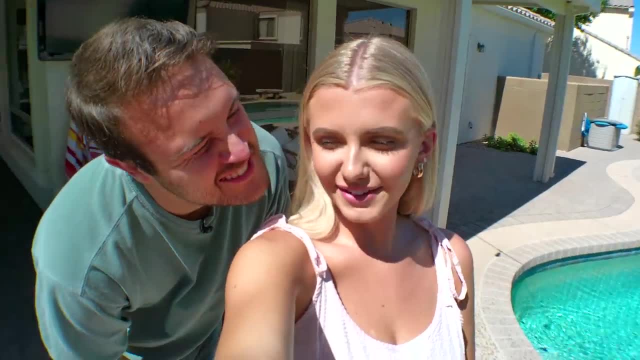 I would like to say that I don't know how this is gonna turn out. I hope it turns out well. How do you feel about me using this camera to shoot my next YouTube video? I don't think that's a good idea. I haven't seen the footage yet. 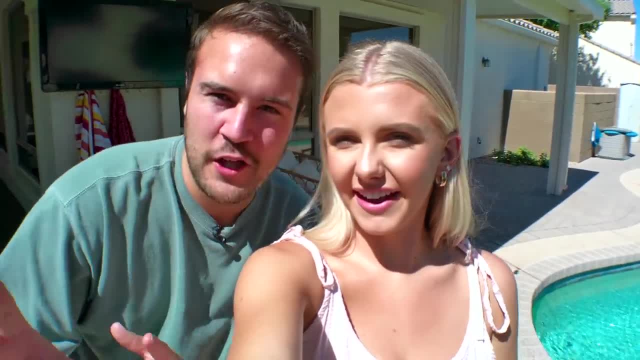 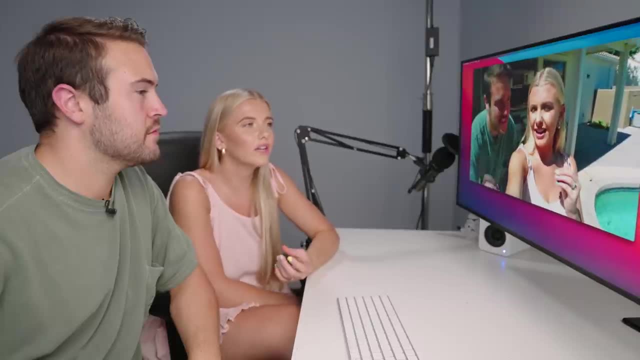 but I just can't imagine. I just can't imagine this. I feel like the colors look okay. I feel like they're bad, Really Okay. let's see how this footage looks. As far as quality goes, I would highly argue that it's 4K. 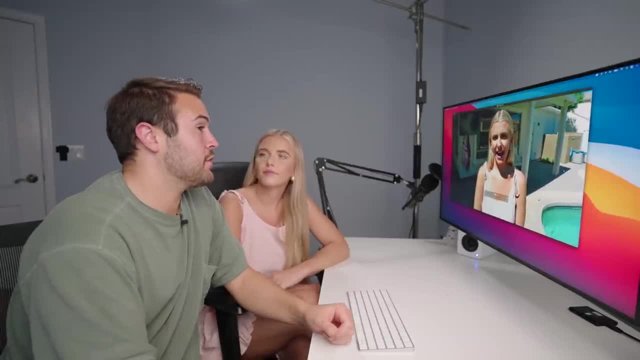 It doesn't look 4K at all. Not at all, Not at all. It's not good, but for a hundred bucks do you think it's worth it? I'd have to see more clips, but I just-. I don't think you're in focus right here either. 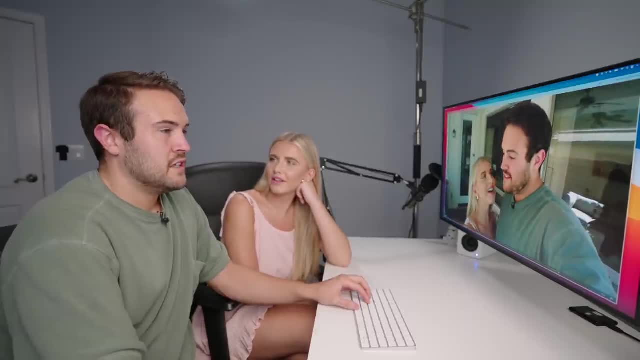 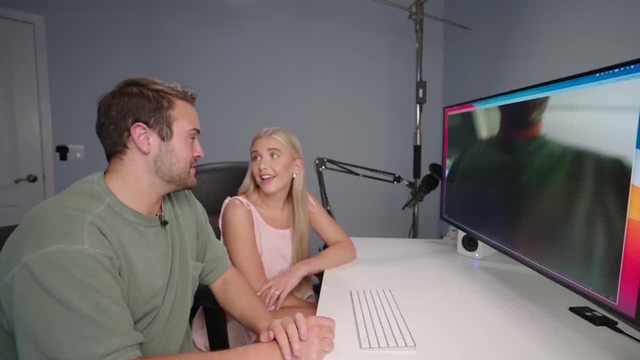 The background's in focus, So you think you can just not be too close to the camera. I don't know. Well, now I need to shoot a full YouTube video, A full YouTube video on this camera. Actually, Yeah, I'd be interested what it looks like right here. 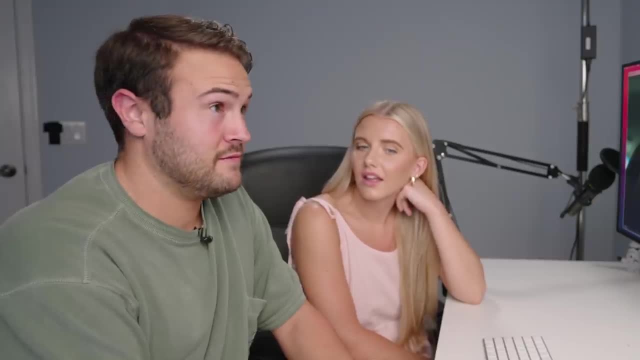 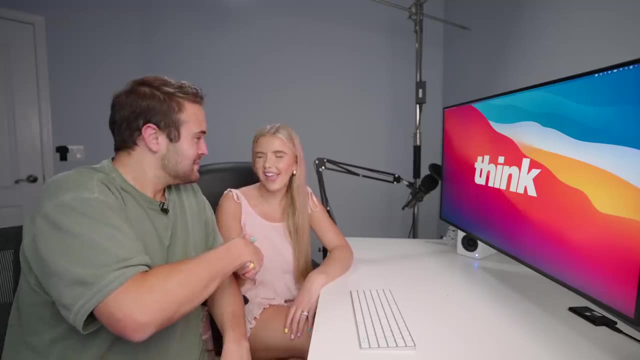 like with a light and everything. I'm gonna try and make it look as good as I can with all my lights, mics, everything. Thank you for being in my video. You're welcome, sir. You know where to find me. 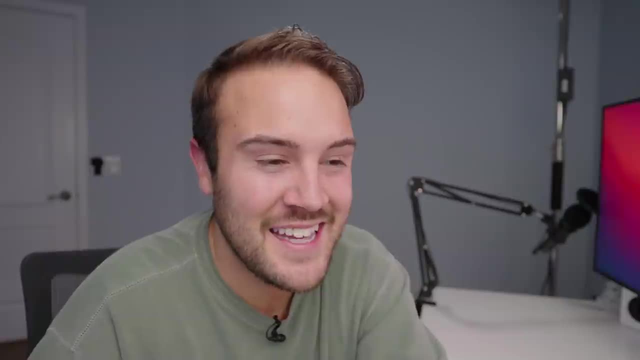 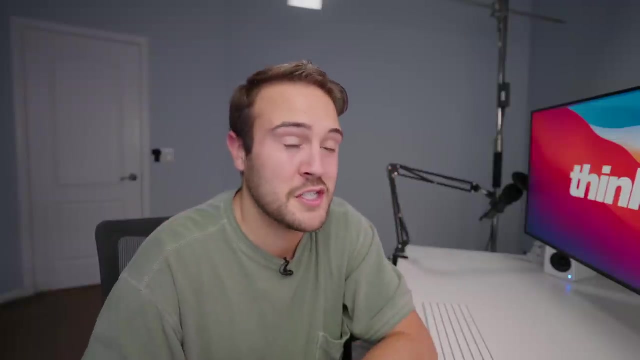 All right, now is the time to shoot my YouTube video using this camera. It's not the best quality at all, but, crossing my fingers, I'm hoping that this video project turns out. okay, Let's just do it. I started to set up the camera, lights, microphone. 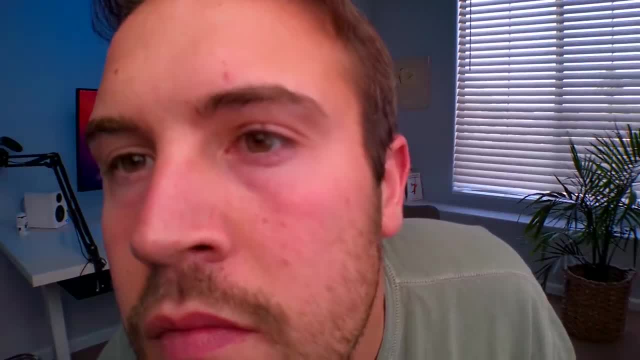 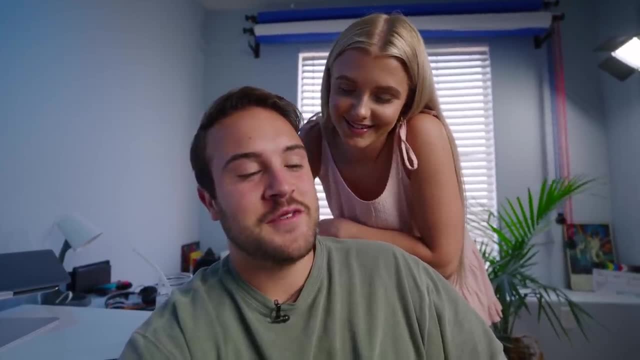 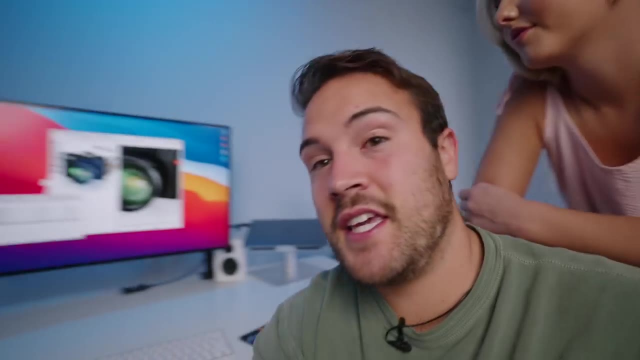 but in doing all of that I found out something about this camera. There's one really bad thing about this camera, Just one: It doesn't autofocus And you can't manually focus either. I tried every setting. I even went back to the Amazon listing here. 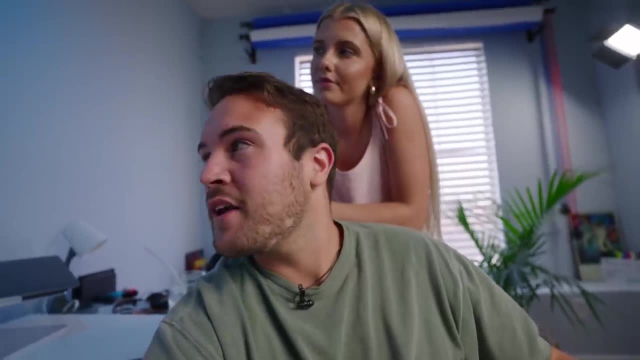 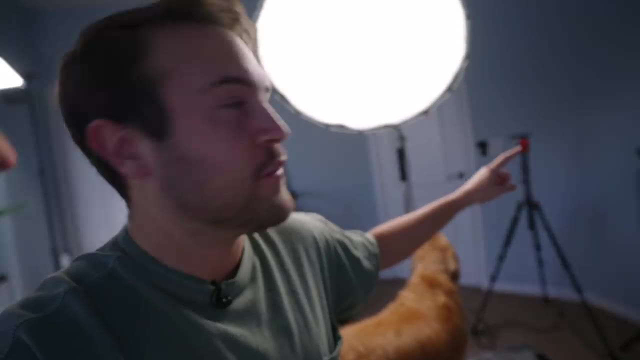 I thought it did say something about autofocus when I bought the camera, but I'm looking at it now and I don't see it. I thought you said it was digital focus. That's not a thing, Ow, The camera's gonna be way over there. 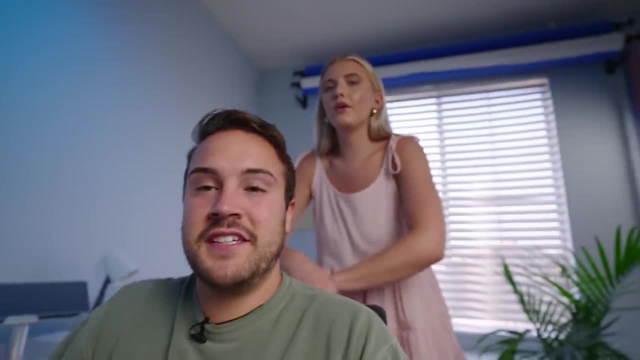 I have to sit way over here and it just looks kind of funky, Oh, in order for it to be in focus. It's like my books back here are in focus, but I'm not totally in focus, So I just don't know what to do. 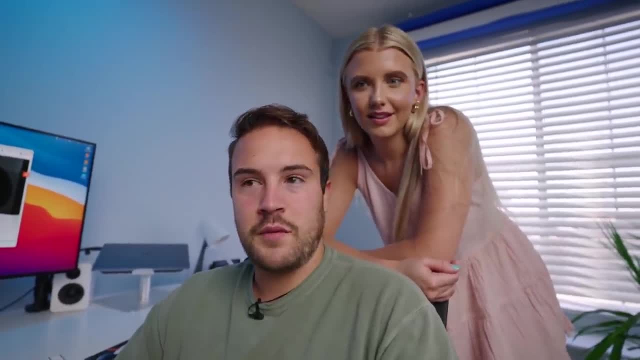 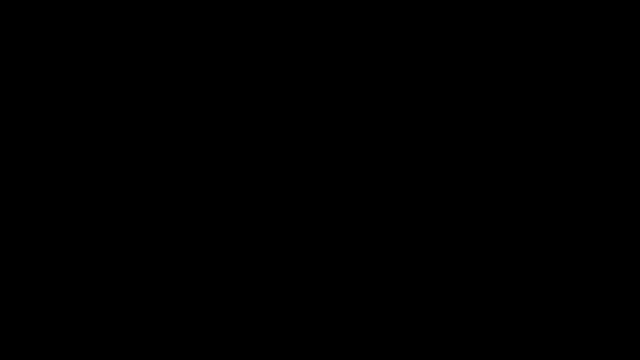 I have to shoot the video, though. Why? Because I told people I would. I committed to this. Is Sean okay with that? Don't know. I don't think you should do it. I really don't, actually don't. My wife thinks that I shouldn't shoot the video on this. 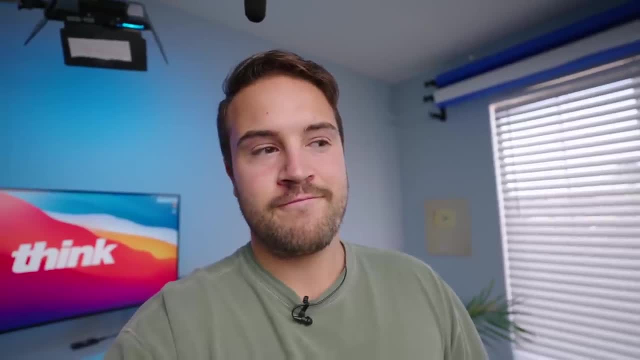 but I told you guys I was gonna do it, So I'm gonna do it, And that's what I did. I pressed record And 20 minutes later I finished filming the video And I'll see you guys in the next video. 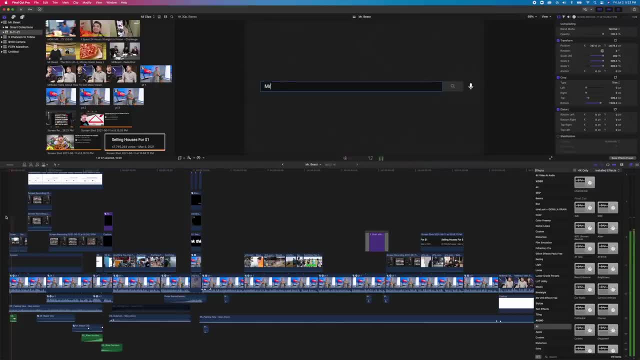 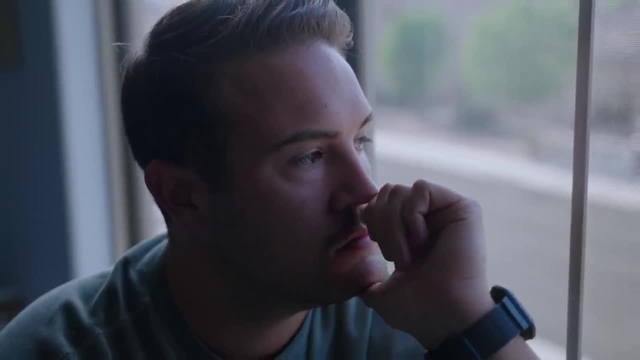 And all I had to do now was edit the video. I kept telling myself that if the content was good enough, then people wouldn't care about the video quality. Even with my positive self-talk, deep down I knew I was still scared. 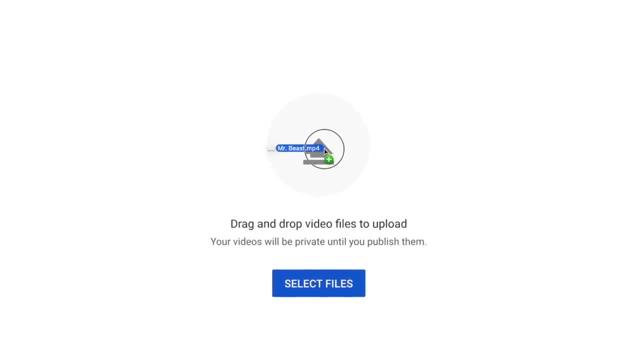 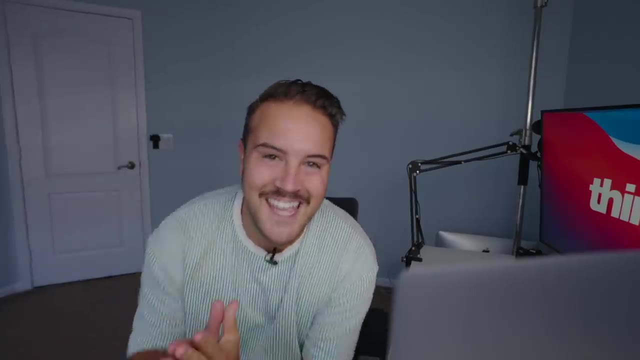 But, regardless of my fears and without telling my boss, I uploaded the video to YouTube. It was time to see if the people would notice. Whew, today is the day. To be honest, I'm a little bit nervous. The video dropped this morning. 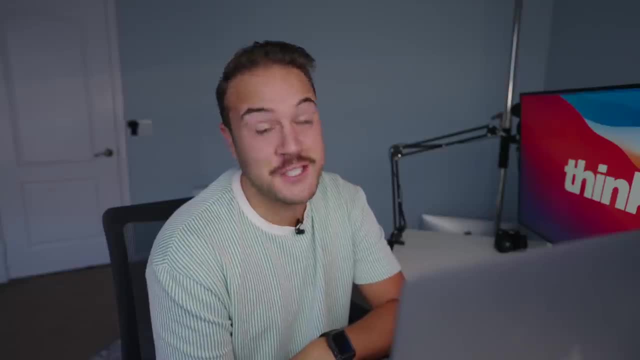 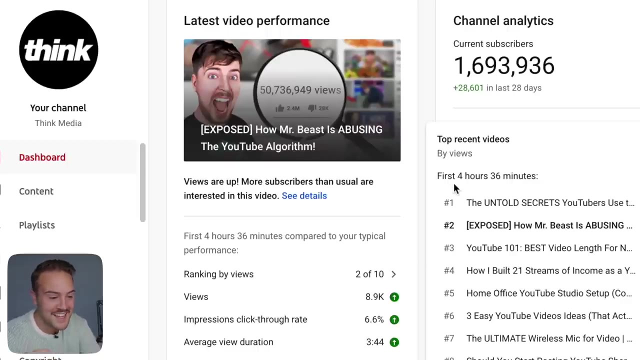 Time to see if this video is performing well and check out the comments. Let's just get right into it. So far, we can see that it's ranking second of 10. within the first four hours: 8.9 thousand views. That's really, really good. 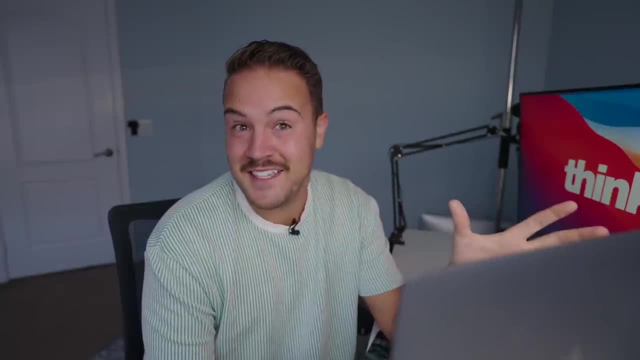 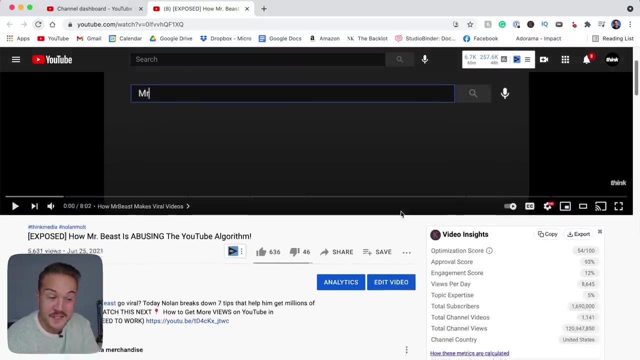 Now for the moment of truth. Let's take a look at the likes, dislikes, as well as the comments, And hopefully I don't get roasted too hard, Let's just get right into it. So here we are: 636 likes and 46 dislikes. 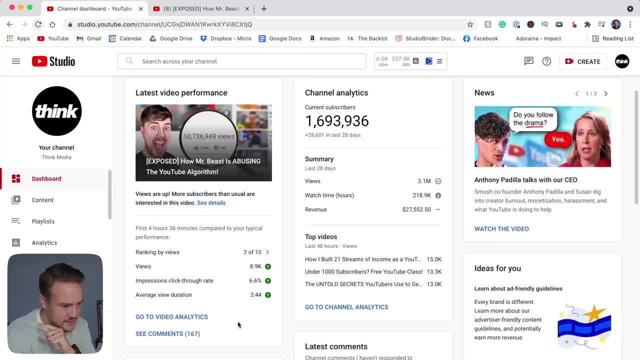 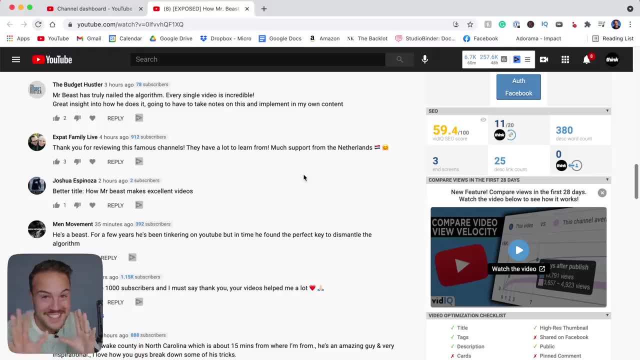 That's pretty good, But really what I'm wondering is the comments. There is 167 comments. All right, let's check these out. I'm only like 10 comments and we have a lot more to go, But so far zero comments about the video quality.